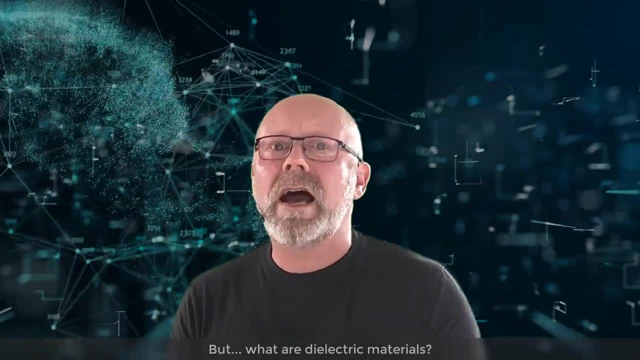 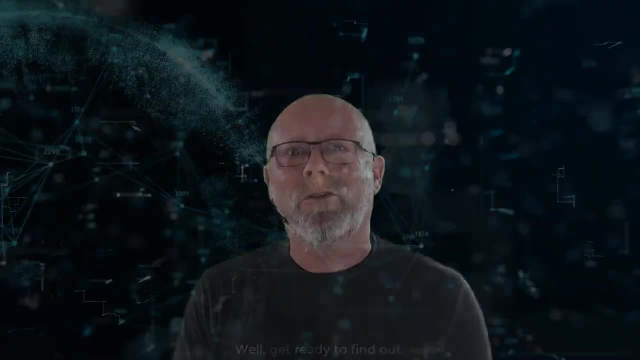 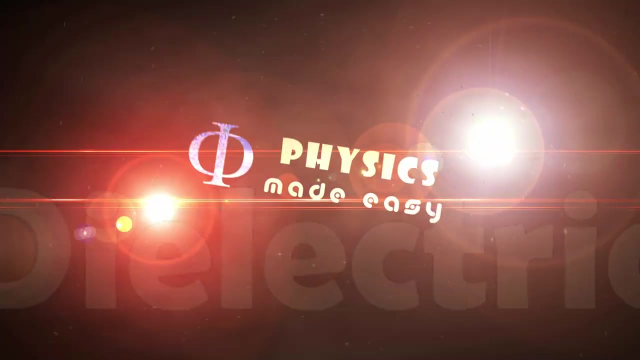 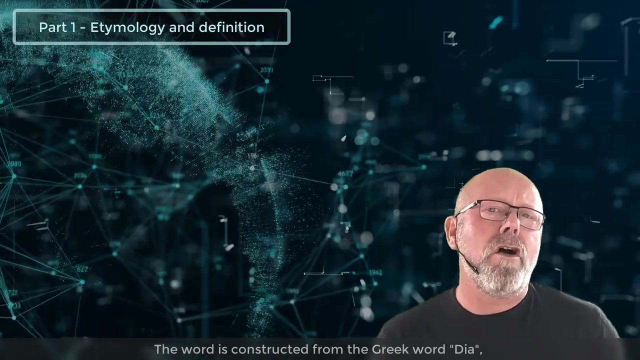 without dielectric materials. But what are dielectric materials? What does the word dielectric even mean? Well, get ready to find out. Let's look at the word itself: dielectric. The word is constructed from the Greek word dia, that means passing through, And electric. well, that refers to. 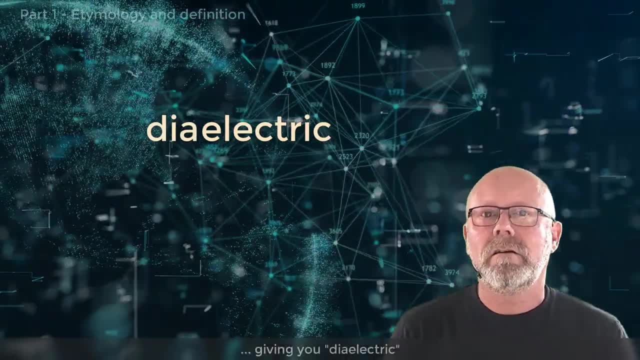 electrical energyification, So dielectric And dielectric. well, that refers to electrical energyification, So dielectric And dielectric. And dielectric Well, that refers to electrical, electric fields giving you dia-electric. This term was proposed by a scientist and philosopher from the 19th century, William. 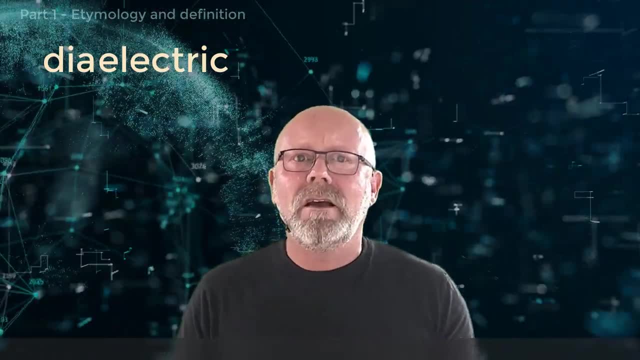 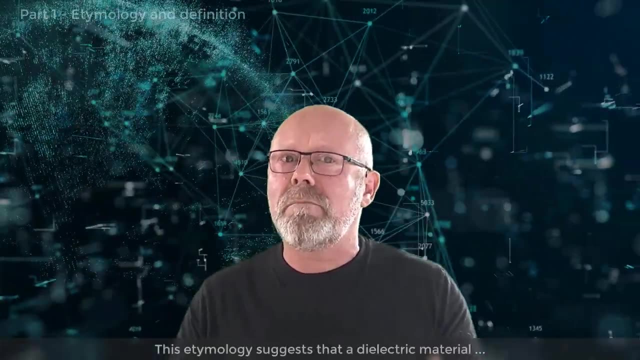 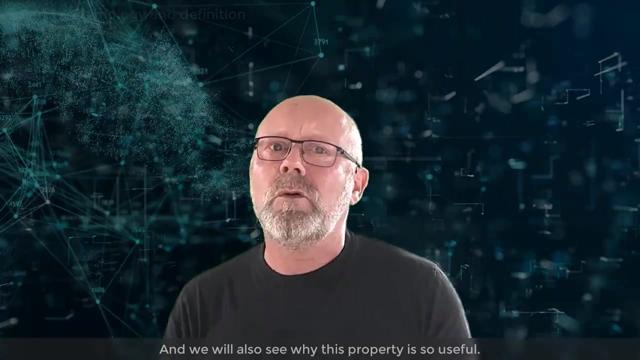 Wewell. Dia-electric is difficult to spell, so with time naturally it compressed into the word dielectric. This etymology suggests that a dielectric material is a material that allows electric fields to pass through it. That is what we will discuss in this video, and we will also see why this property is. 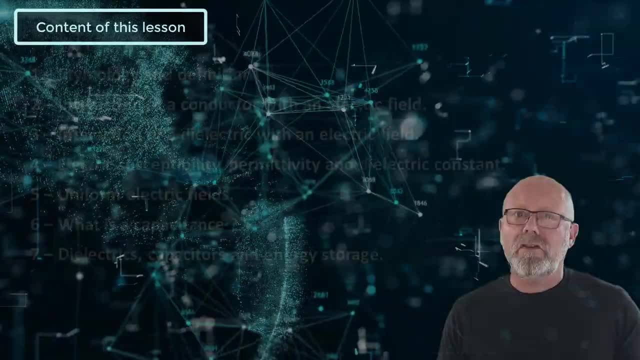 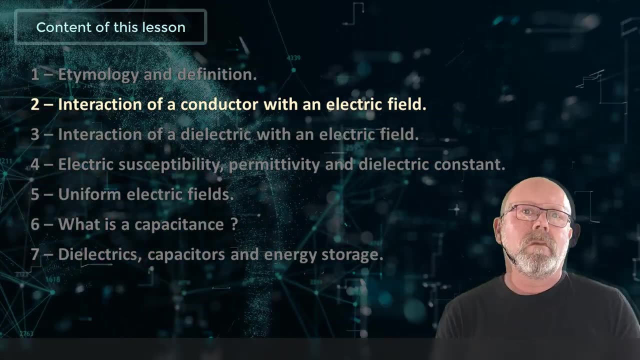 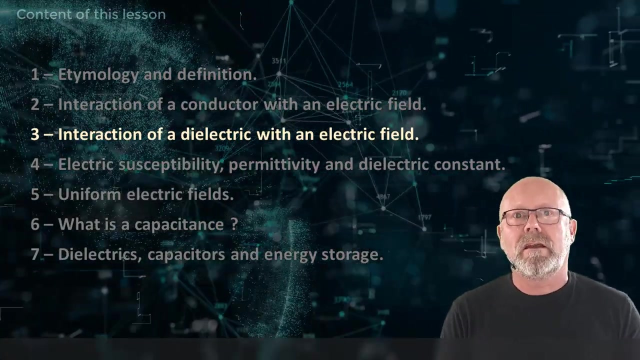 so useful. First we will look at what happens to an electric field when it is applied to a conducting material like a piece of metal. Then we will look at what happens to that electric field when it is applied to a dielectric material like a piece of ceramic. 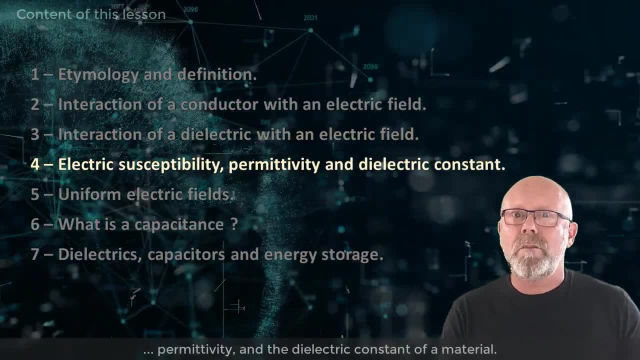 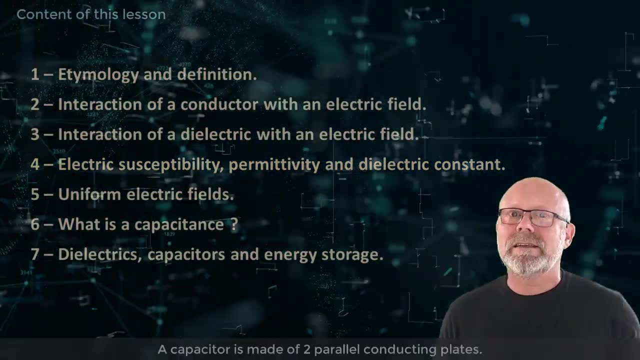 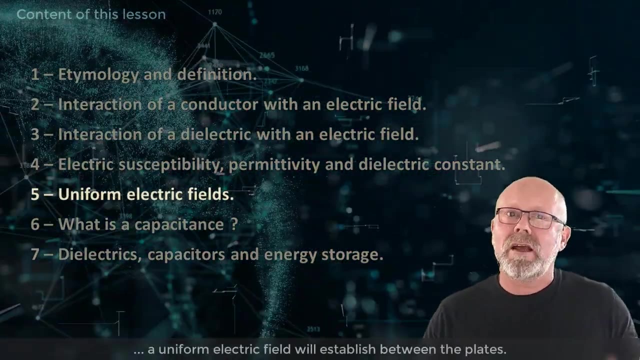 That's where we will discuss the concept of electric susceptibility, permittivity and the dielectric constant of a material. Dielectrics are used mostly in capacitors. A capacitor is made of two parts. They are parallel conducting plates. If the plates are connected to a DC source, a uniform electric field will establish between. 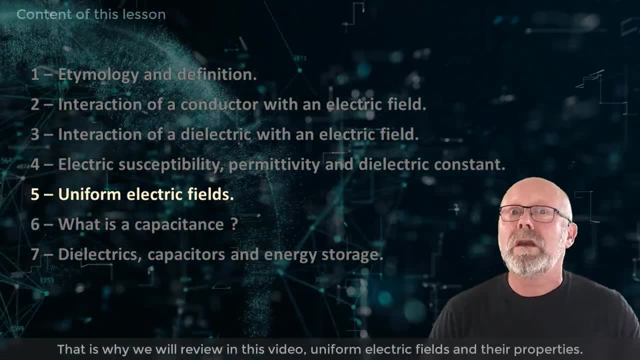 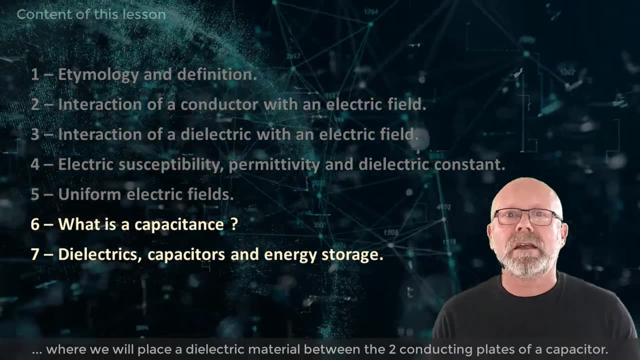 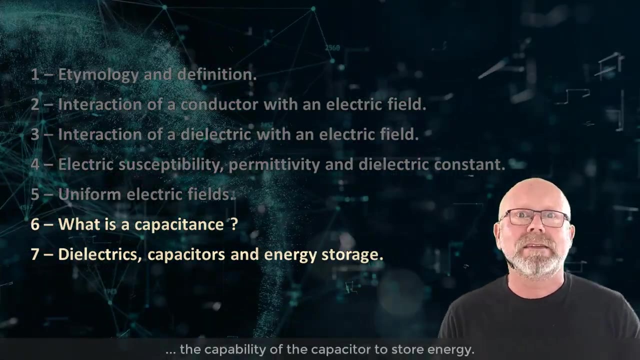 the plates. That is why we will also review in this video uniform electric fields and their properties. Everything will come together in the last section of the video, where we will place a dielectric material between the two conducting plates of a capacitor. By doing so we will realize how that improves the capability of the capacitor to store energy. 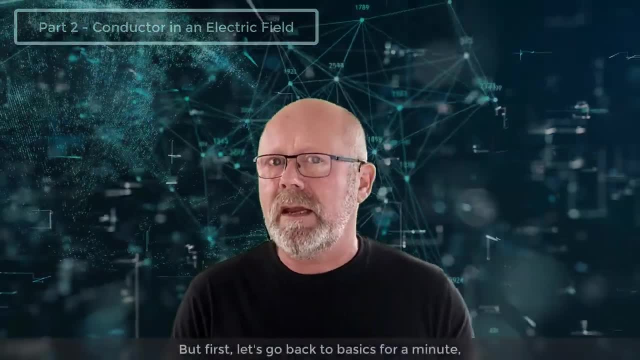 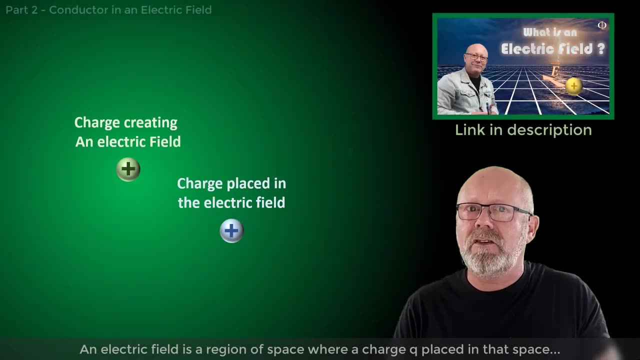 But first let's go back to basics. for now, To explain the basics for a minute by defining what an electric field is. An electric field is a region of space where a charge, Q, placed in that space, experiences a force. F equals Q by E, where E is the strength of the field or, if you prefer, the force. 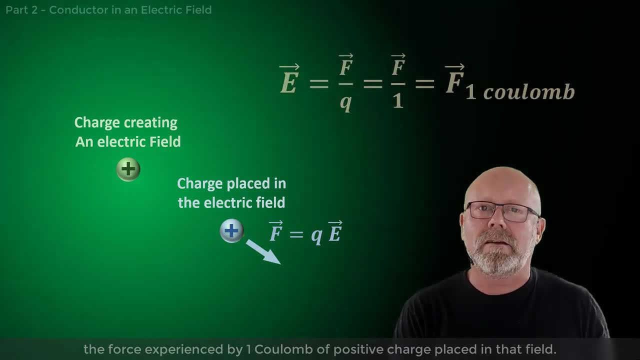 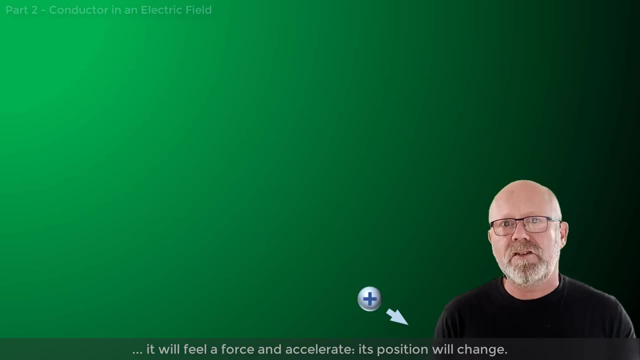 experienced by one coulomb of positive charge placed in that field. If I place a charge free to move around in an electric field, it will feel a force and accelerate. It's position will change. Now let's imagine I place a piece of metal in a uniform field of strength E I will place 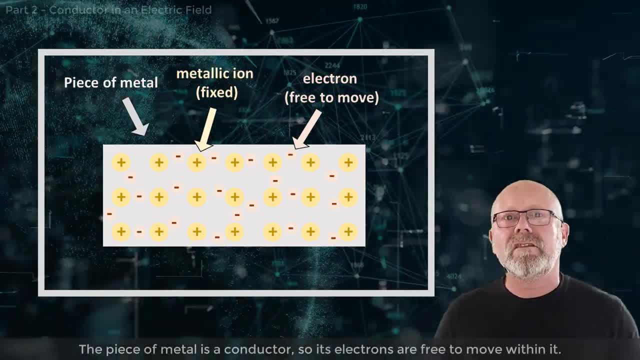 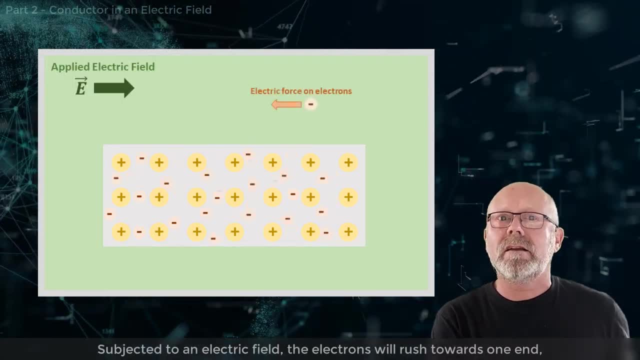 a piece of metal in an uniform field of strength E. Let's imagine I place a piece of metal in an uniform field of strength E. Now I place, The piece of metal is a conductor, so electrons are free to move within it. Subjected to an electric field, the electrons will rush towards one end, leaving the other. 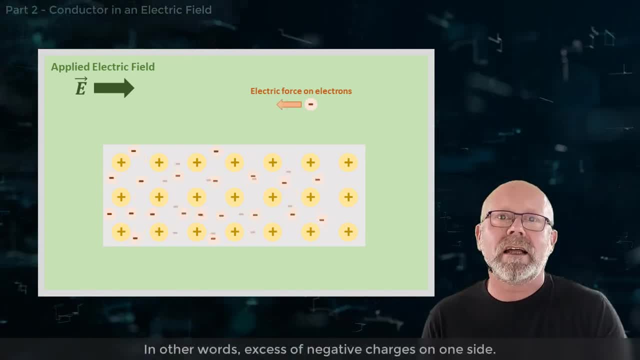 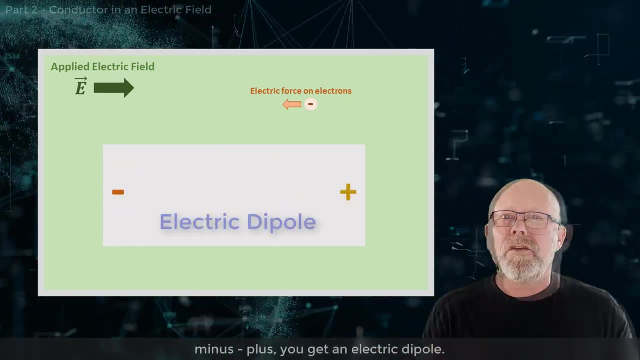 end with a deficit of electrons, In other words, excess of negative charges on one side, excess of positive charges on the other. minus plus, you get an electric dipole. The trick lies here. This new dipole generates its own electric field, E' that opposes the applied electric. 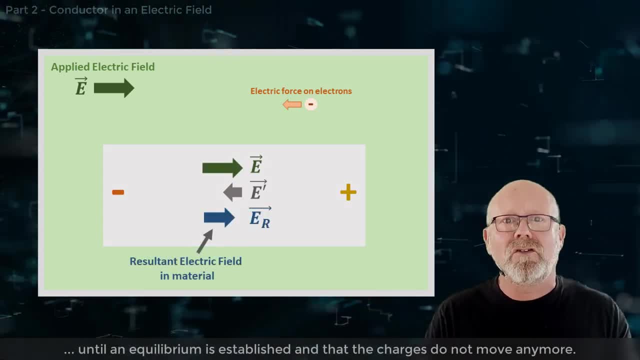 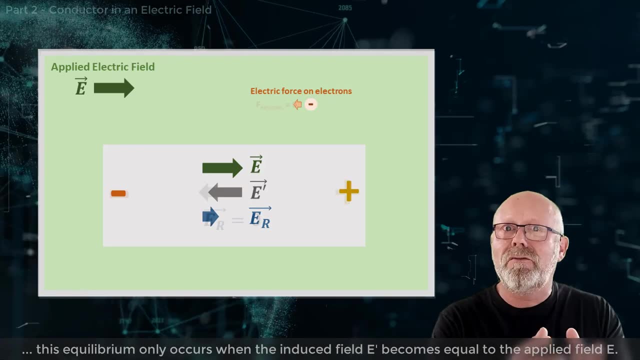 field E until an equilibrium is established and that the charges do not move anymore, Because the charges are totally free to move. this equilibrium only occurs when the induced field E' is equal to the applied field E, So the resultant field in the material is: 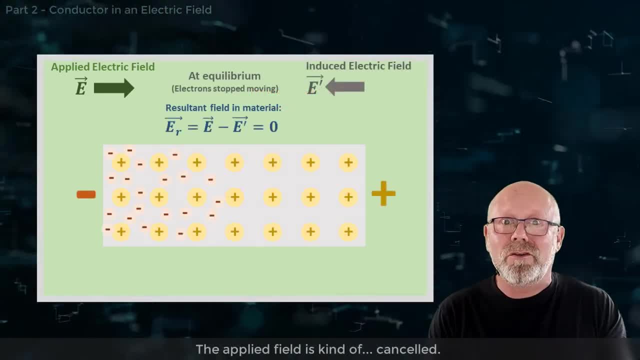 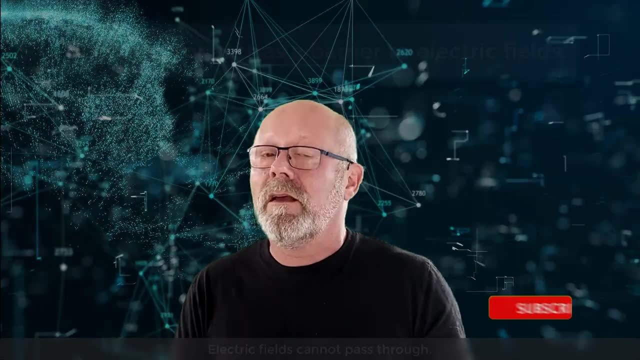 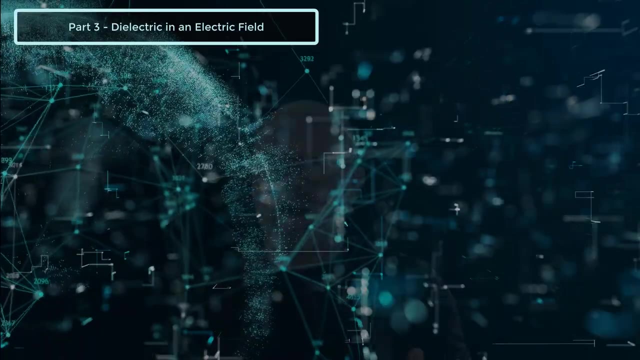 zero, The applied field is kind of cancelled. a conducting material acts as a barrier to electric fields. Electric fields cannot pass through And, by the way, this is the principle behind Fahady's case. Now let's expose a dielectric material to the same field, E. 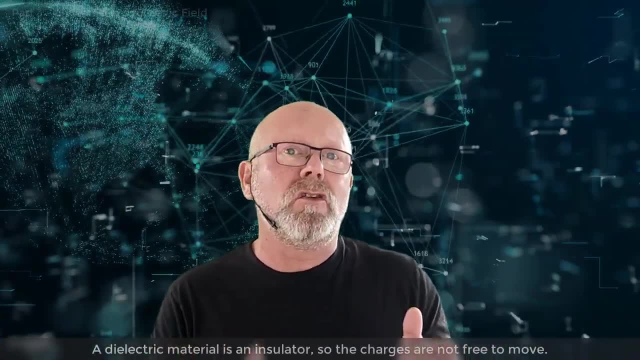 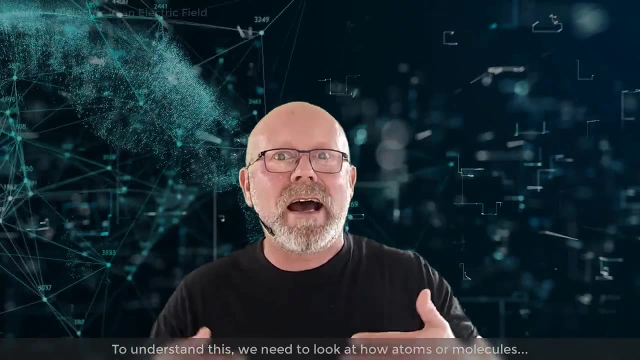 A dielectric material is an insulator, so the charges are not free to move, Or maybe a little bit, And this little bit is crucial. To understand this, we need to look at how atoms or molecules interact with an applied electric field. 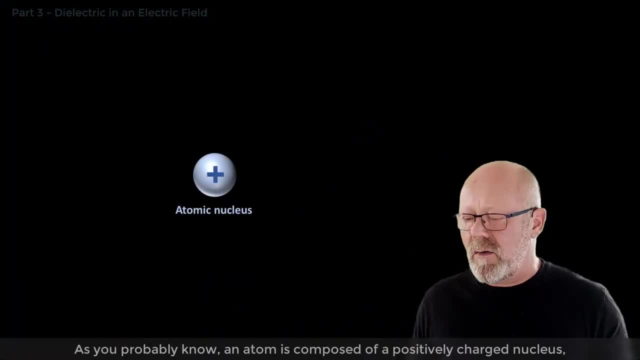 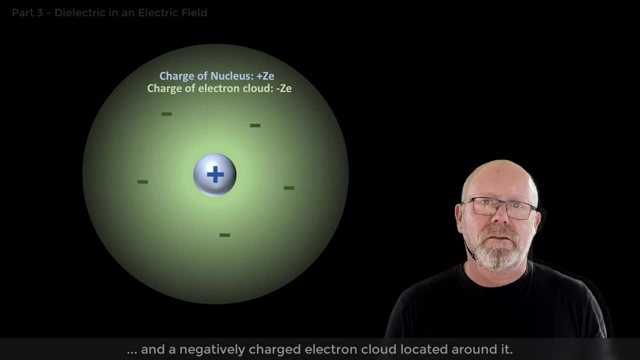 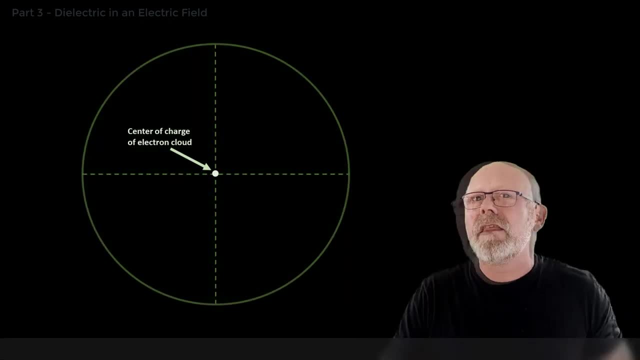 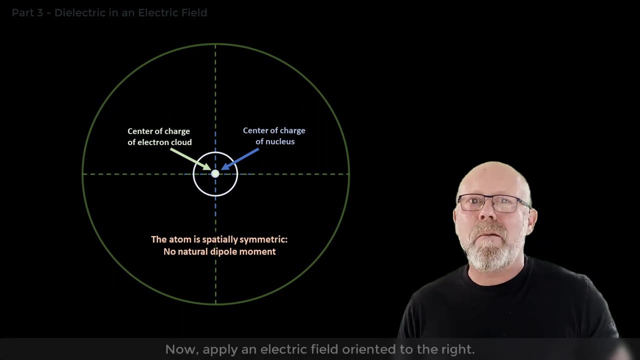 If you look at the center of charges for the electron cloud, which is negative, and the center of charges for the nucleus, which is positive, they are in the same position. Yes, an atom is symmetric. Now apply an electric field oriented to the right. 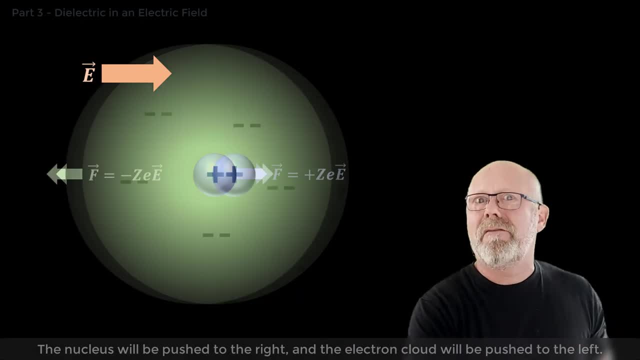 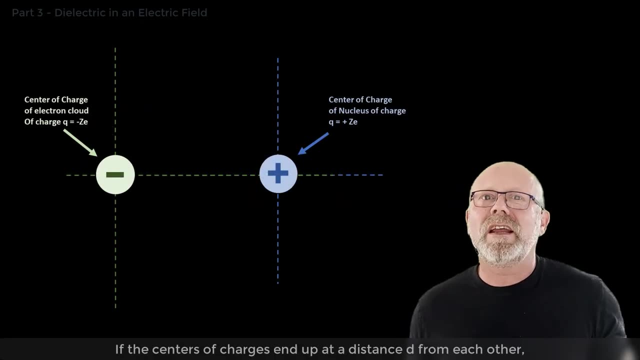 The nucleus will be pushed to the right and the electron cloud will be pushed to the left. The positive and negative center of charges dissociate and move away from each other, creating a dipole. If the center of charges end up at a distance d the positive and negative center of charges, 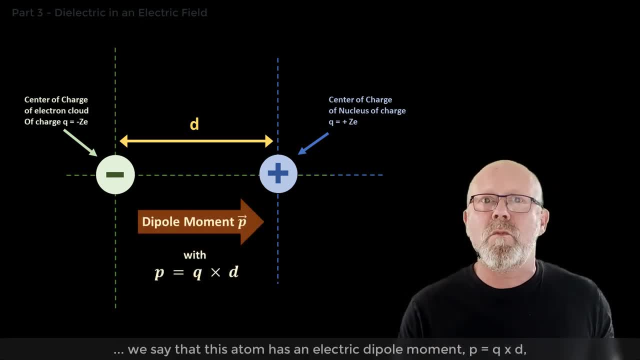 move away from each other, creating a dipole. We say that this atom has an electric dipole moment. p is equal to q multiplied by d, where q is the charge of the electron cloud that was displaced. Note that p, the electric dipole moment, is a vector. 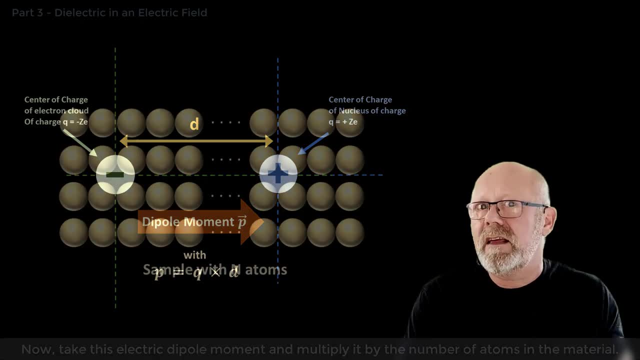 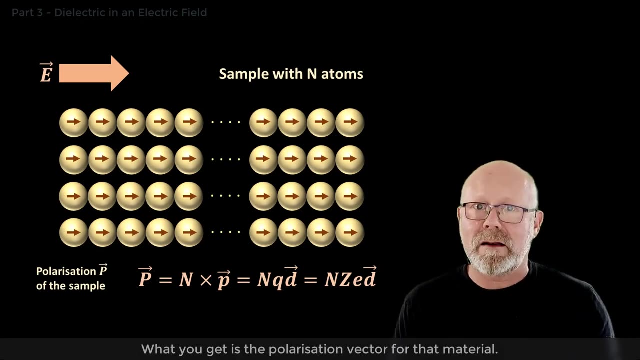 It has a direction. The atom is polarized. Now take this electric dipole moment and multiply it by the number of atoms in the material. What you get is the polarization vector for that material. This type of polarization is called electronic polarization. Other types of polarizations can also be called electronic polarization. 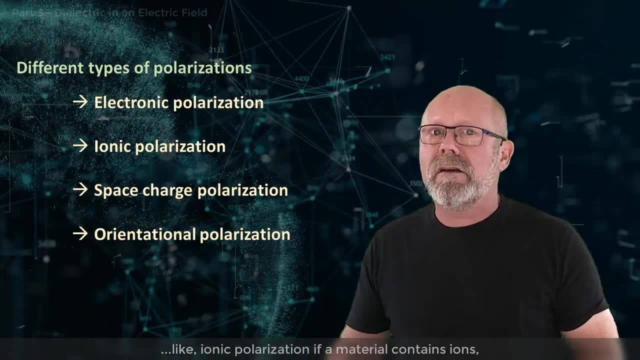 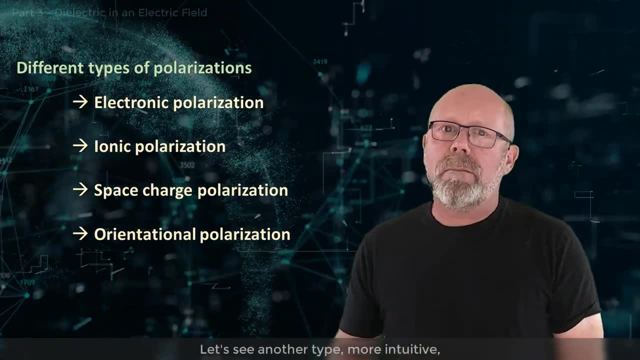 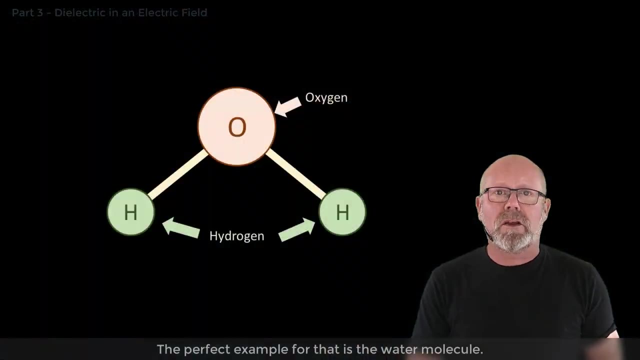 Like ionic polarization if a material contains ions, And space charge polarization if it contains a few free charges. Let's see another type, more intuitive, called orientational polarization. The perfect example for that is the water molecule. In a water molecule, the oxygen atom is more electronegative than the hydrogen atoms. 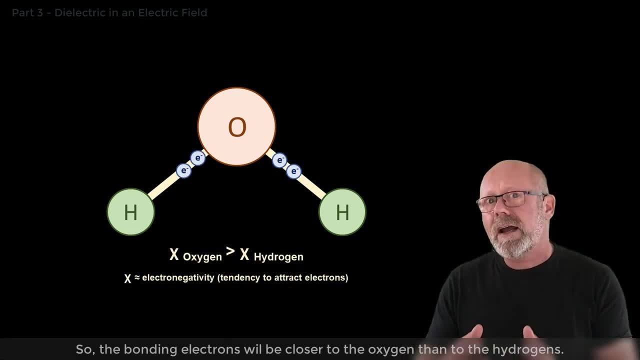 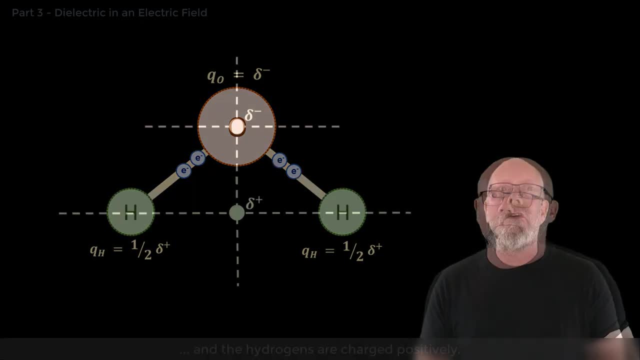 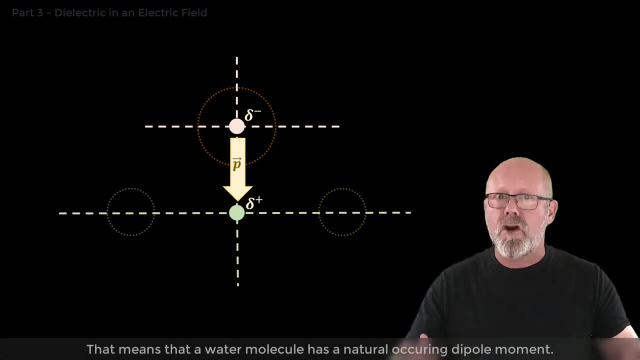 So the bonding electrons will be closer to the oxygen than to the hydrogens. Consequence: The oxygen is charged negatively and the hydrogens are charged positively. The positive and negative centers of charges are not at the same position. That means that a water molecule has a natural occurring dipole moment and thus a polarization. 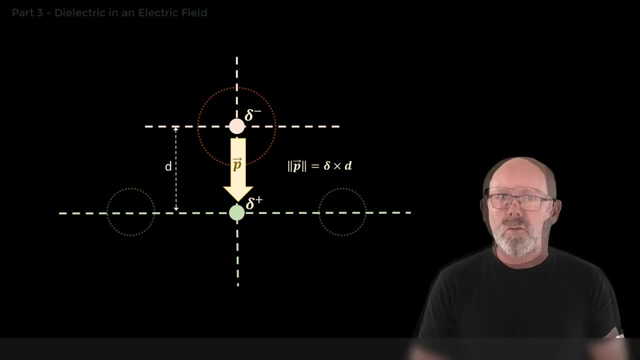 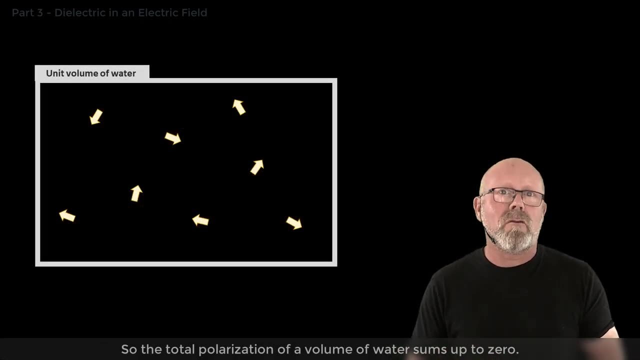 That is why, in chemistry, water is said to be a polar molecule. In the absence of an electric field, water molecules are oriented randomly, So the total polarization of a volume of water sums up to zero. So the total polarization of a volume of water sums up to zero. 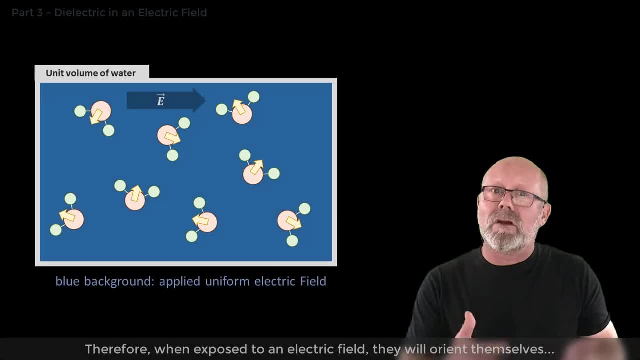 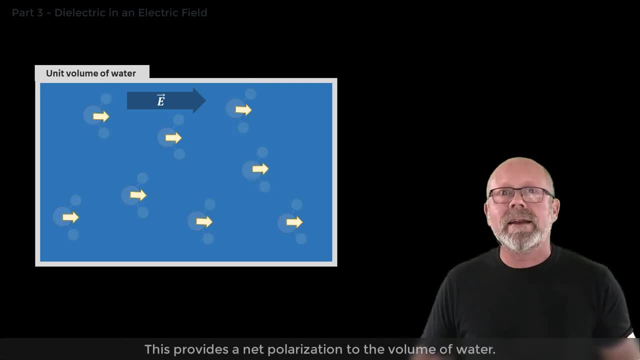 So the total polarization of a volume of water sums up to zero. Therefore, when exposed to an electric field, they will orient themselves so that the dipole moment vectors align with the direction of the field. This will provide a net polarization to the volume of water. 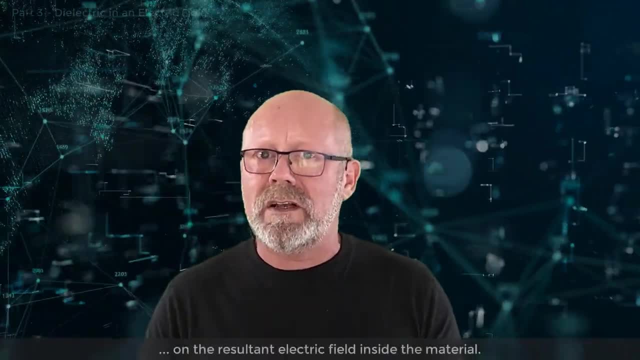 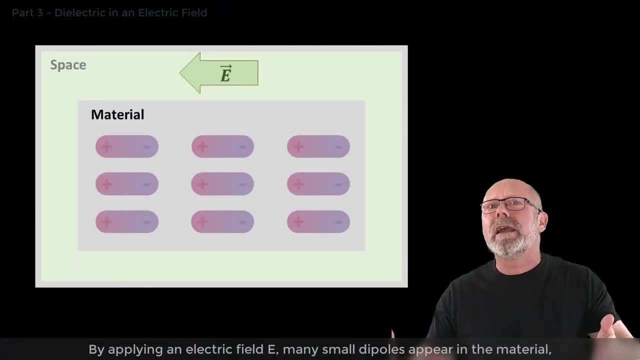 Whatever the type of polarization, it will have an effect on the resultant electric field inside the material. Look at this: By applying an electric field E, many small dipoles appear in the material, each inducing their own electric field in opposite direction to E. 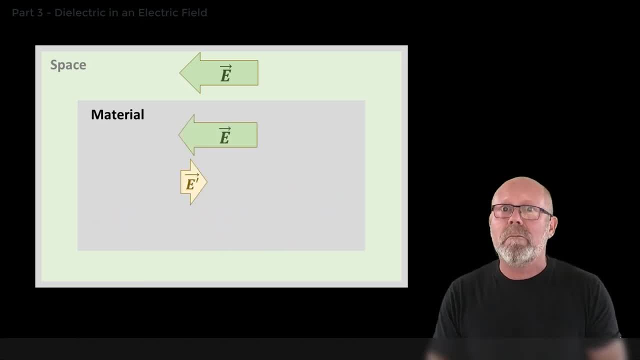 But what happens when you apply an electric field E to a known particle in the material, to a global induced electric field E' that opposes the applied electric field E. After a transitory period an equilibrium forms. The resultant electric field in the material is the vector sum of the applied electric. 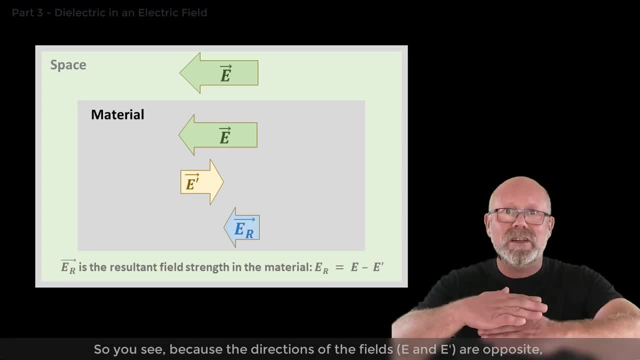 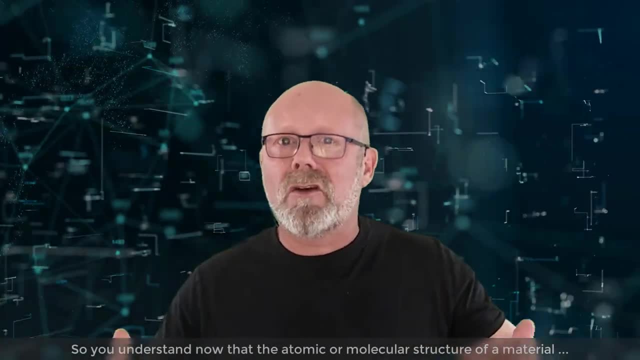 field and the induced electric field, that is E minus E'. So you see, because the directions of the fields are opposite, the resultant field within the material is weaker than the applied field. So you understand now that the atomic or molecular structure of a material is different from. 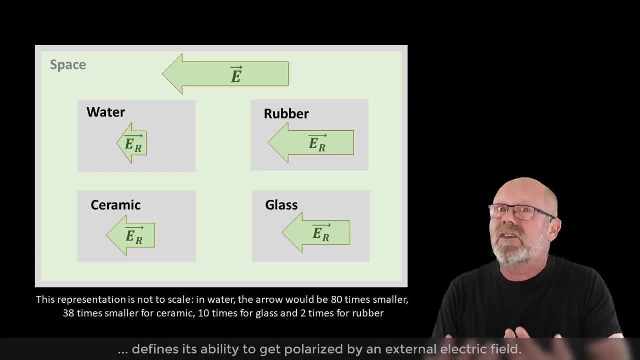 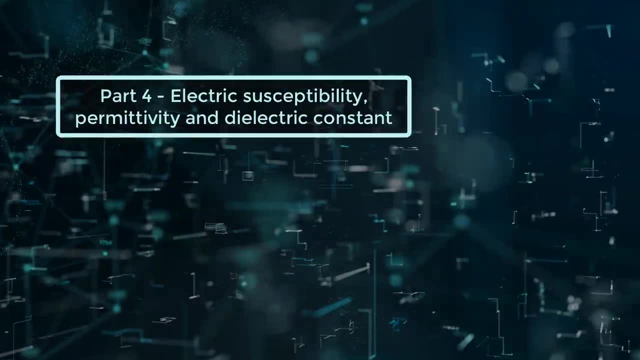 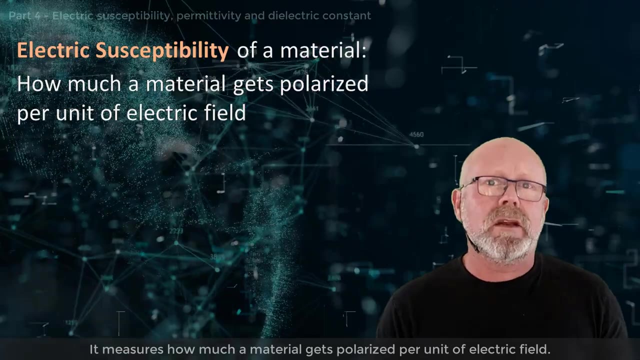 the inducing electric field will define its ability to get polarized by an external electric field and consequently impact the resultant field within it. This property is called the susceptibility of a material. It measures how much a material gets polarized per unit of electric field. 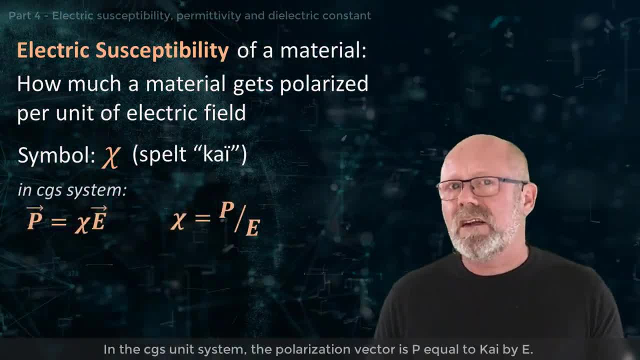 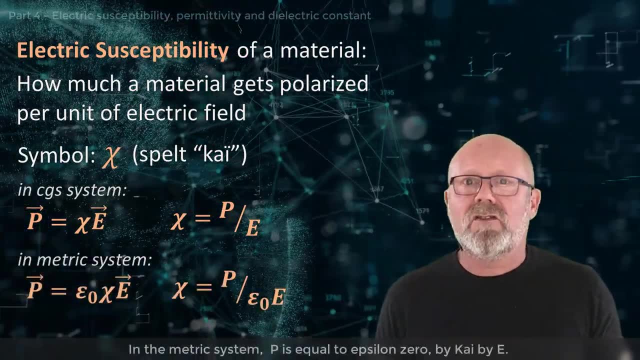 It is represented by the Greek letter chi. In the CGS unit system the polarization of vector is: p is equal to chi by the electric field strength. In the metric system, p is equal to epsilon zero by chi by E, where epsilon zero is called the permittivity of vacuum. 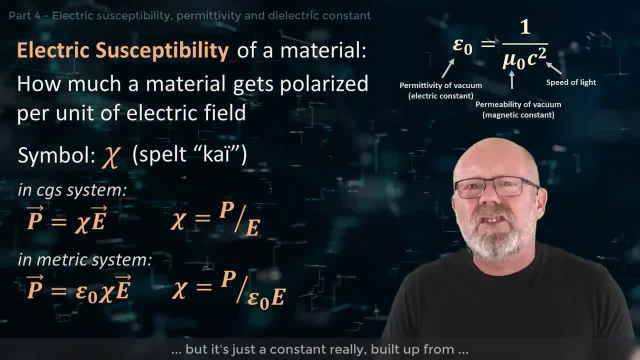 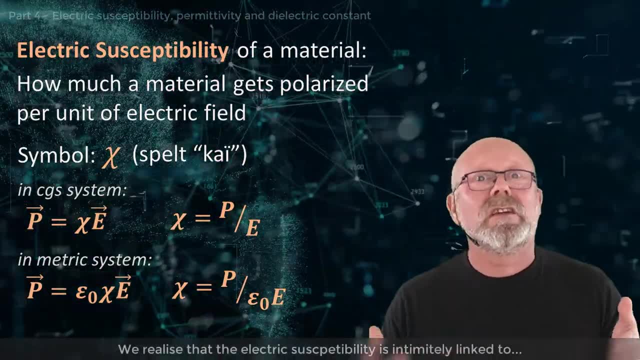 Epsilon zero is there for historical reasons, but it's just a constant, really built up from other fundamental constants related to empty space. So we realize that the electric susceptibility is intimately linked to the ability of a material to weaken the electric field passing through it. 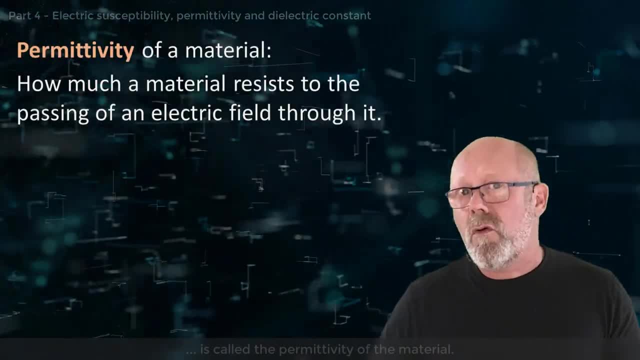 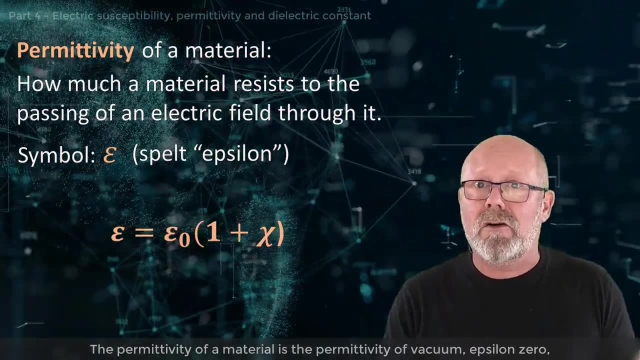 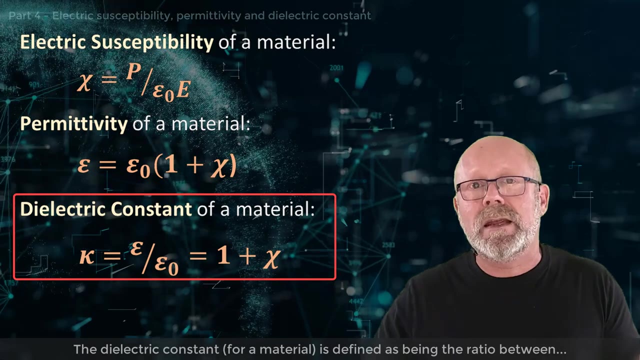 That resistance to letting the electric field pass through is called the permittivity of the material, Epsilon. The permittivity of a material is the permittivity of vacuum- epsilon zero multiplied by one, plus the electric susceptibility, chi. The dielectric constant is defined as being the ratio between epsilon and epsilon zero. 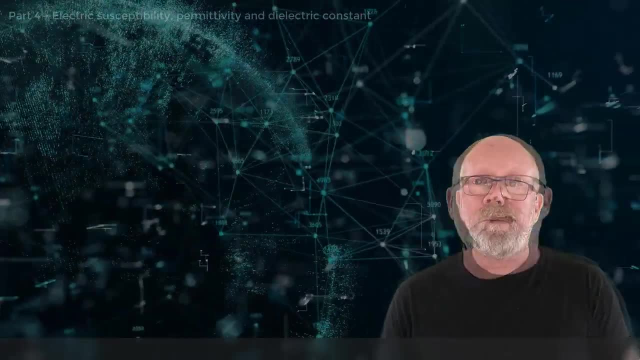 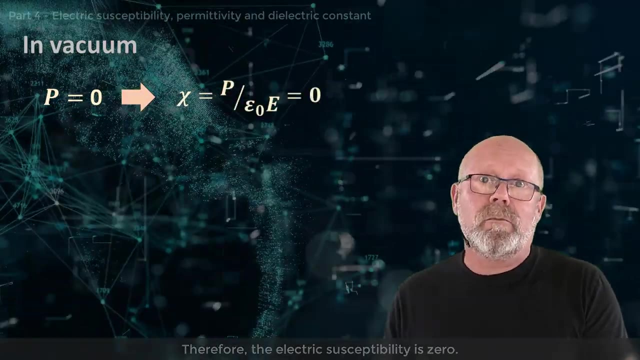 and therefore also equal to one plus chi. Consider vacuum: In vacuum, there's nothing that can get polarized right. Therefore, the electric susceptibility is zero. That means that the dielectric constant is one. That means also that the electric susceptibility is zero. 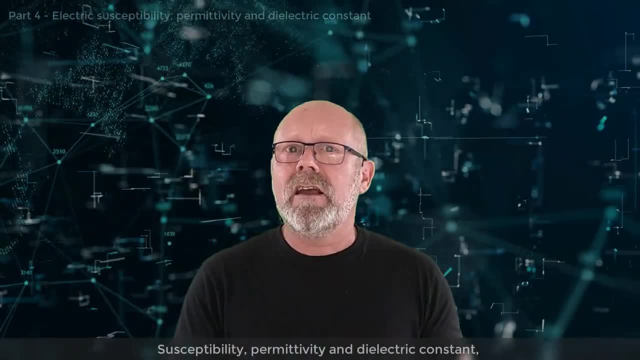 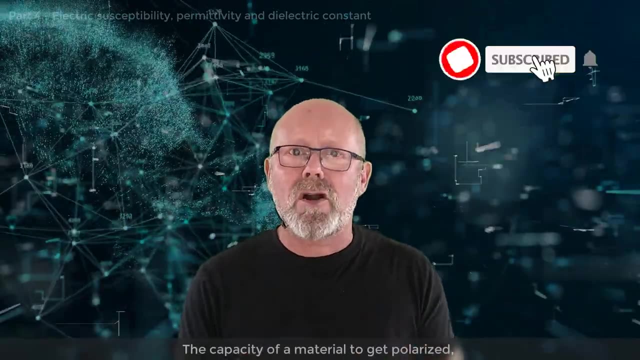 That means also that the permittivity is epsilon, zero Susceptibility permittivity and dielectric constant all mean roughly the same thing: The capacity of a material to get polarized, In other words to oppose an electric field that is applied to it. 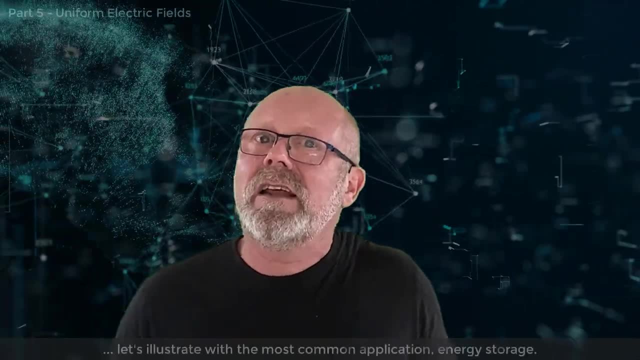 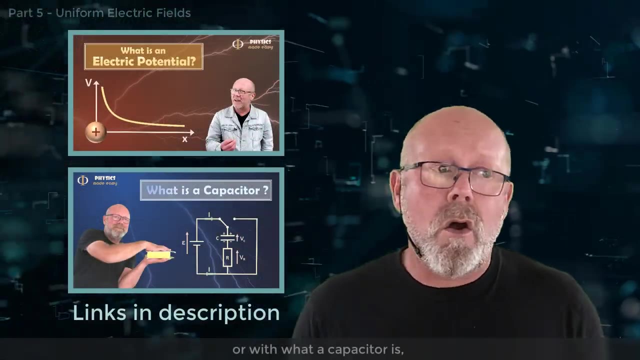 Now that you have a good grasp of what a dielectric material is, let's illustrate with the most common application: energy storage. If you're not familiar with what an electric potential is or with what a capacitor is, I recommend you check these videos before going further. 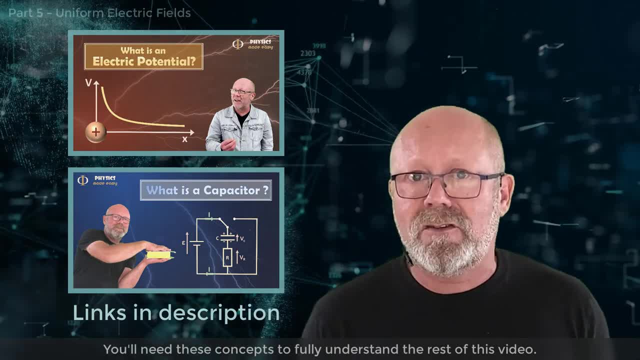 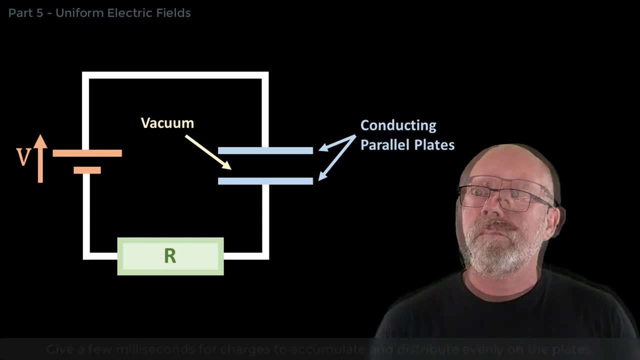 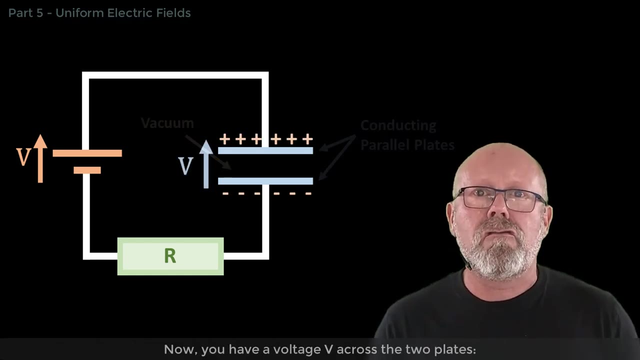 You'll need these concepts to fully understand the rest of this video. Let's look at two parallel plates that I connect to a battery delivering a voltage V, Give a few milliseconds for charges to accumulate and distribute evenly on the plates. Now you have a voltage V across the two plates. 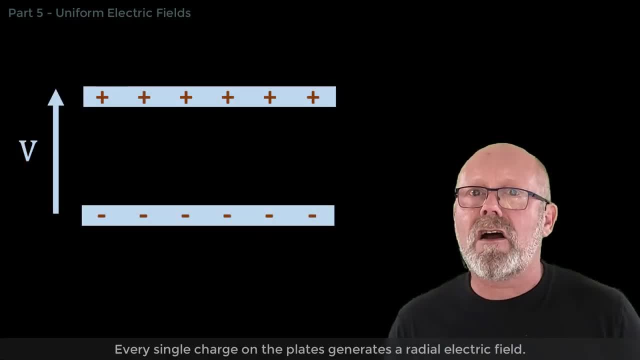 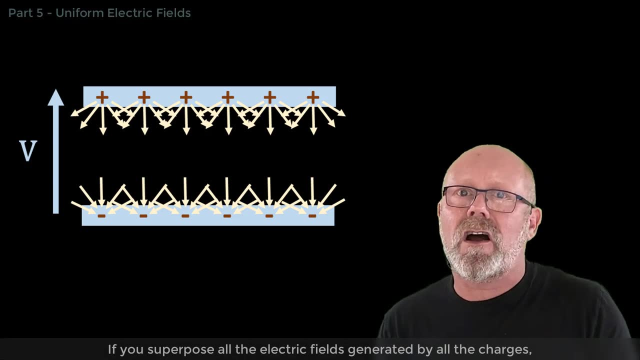 The capacitor is fully charged. Every of the charges on the plates generate a radial electric field. If you superpose it, if you superpose all the electric fields generated by all the charges, you end up with a resultant field E between the plates, which is uniform. 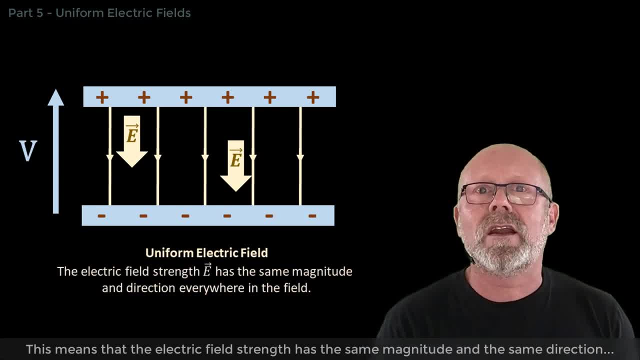 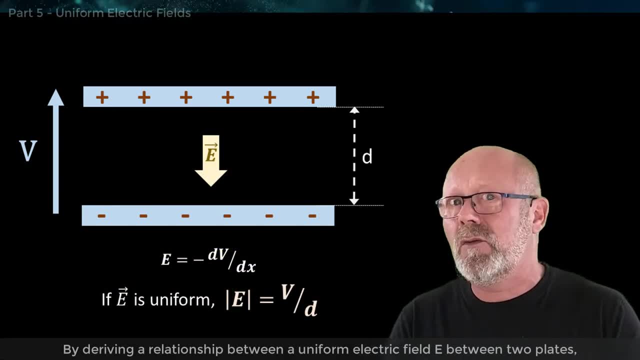 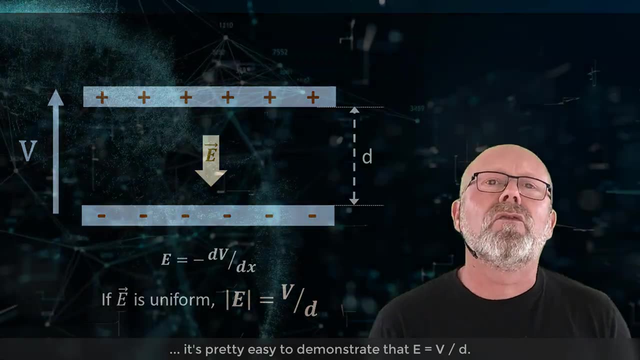 This means that the electric field strength has the same magnitude and the same direction at all points between the plates. By deriving a relationship between a uniform electric field E between two plates which are separated by a distance, d, with a voltage V, it's pretty easy to demonstrate that E is equal to V over d. 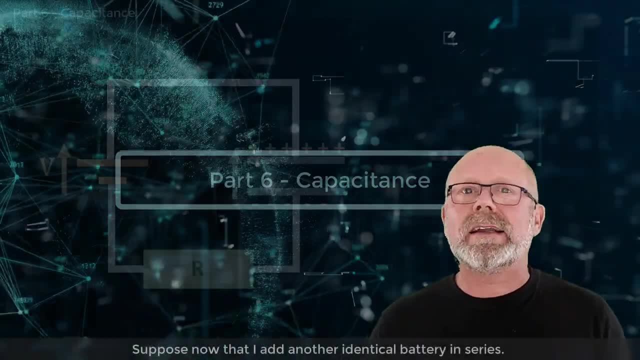 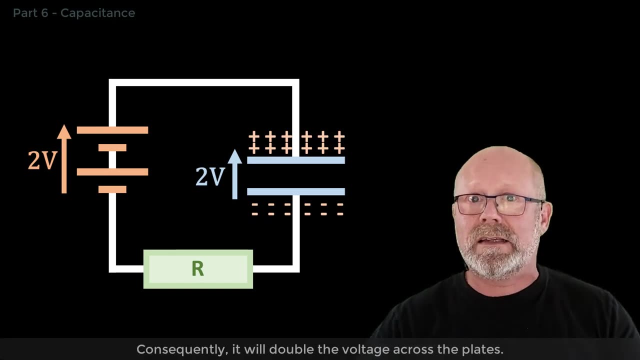 Suppose now that I add another identical battery in series, This will provide enough energy to double the amount of charges on the plates. Consequently, it will double the voltage across the plates. Voltage to a capacitor and the amount of charge on the plates are proportional. 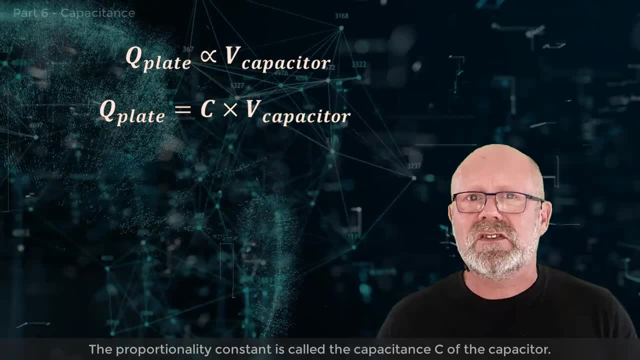 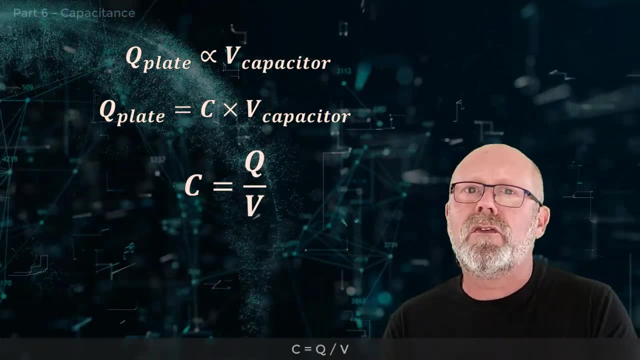 The proportionality constant is called the capacitance C of the capacitor. Q equals C- V Or, if you prefer, C is equal to Q over V. The capacitance tells you how much charge you have And how much charge you can store in a capacitor for each volt you apply to it. 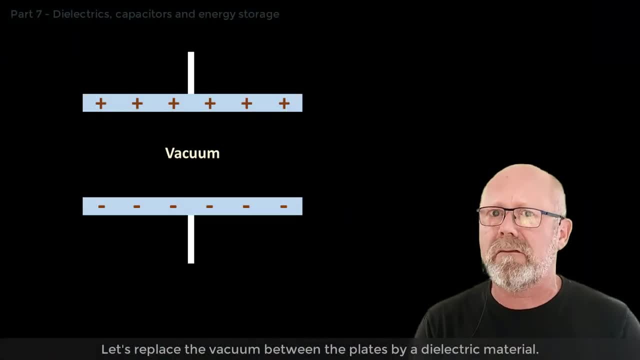 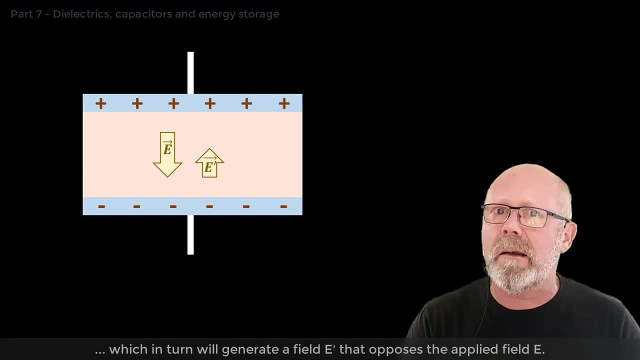 Let's replace the vacuum between the plates by a dielectric material. The applied field will cause a polarization of the dielectric material, which in turn will generate a field E prime that opposes the applied field E. The resultant field between the plates- E minus E prime- is now weaker. 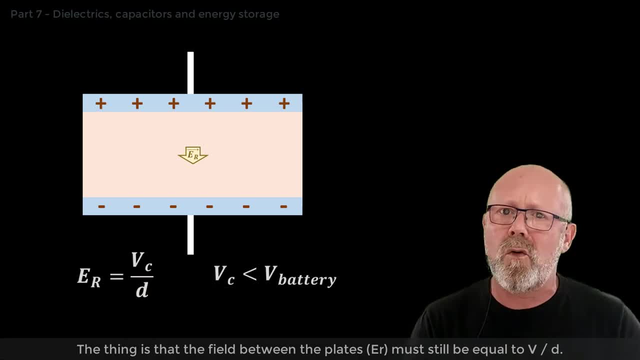 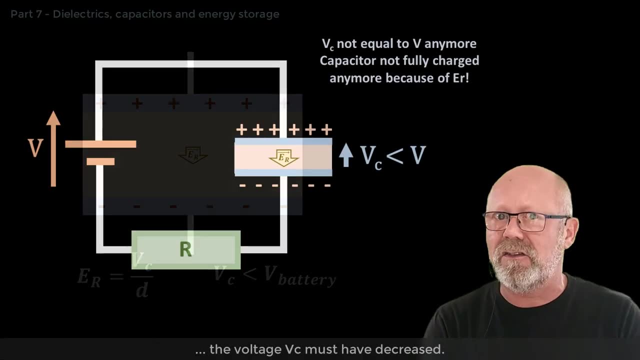 The thing is that the field between the plates must still be equal to V over d. The distance d between the plates hasn't changed, So the voltage V must have decreased. But V is fixed by the battery In order to restore the original voltage V across the capacitor. 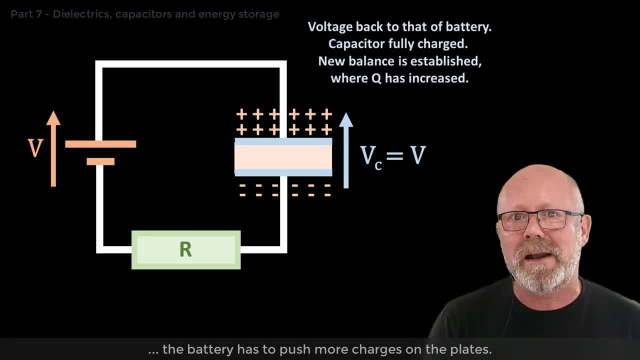 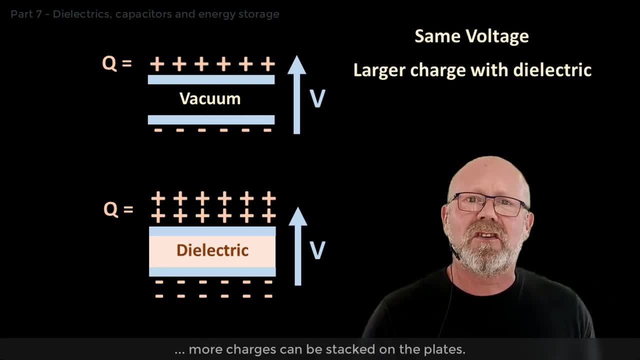 the battery will have to push more charges on the plates. By replacing the vacuum by a dielectric and for the same voltage across the capacitor, more charges can be stacked on the plates. In other words, the capacitance increases. And that's not all.